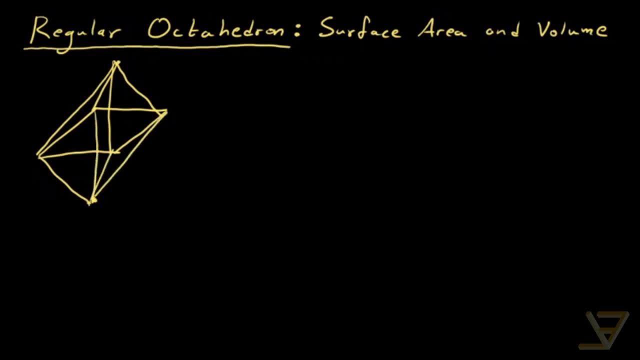 Now what we want to do is find the surface area and the volume of this figure. It's a polyhedron. What we know is that each of the eight triangles is an equilateral triangle And the area of the eight triangles is an equilateral triangle. 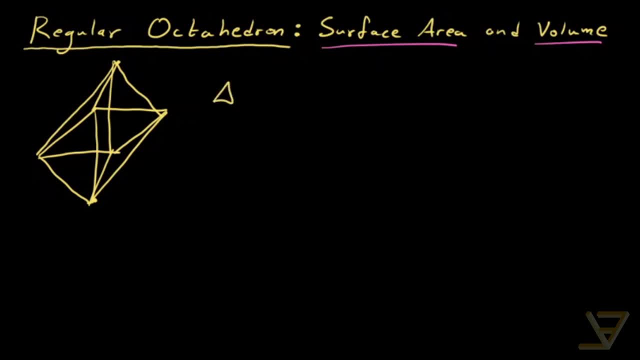 The volume of an equilateral triangle with side length s is equal to square root of three s squared over four. So all we have to do is do eight times the area and we get two square root of three s squared. And that is the area, the surface area of the regular octahedron. 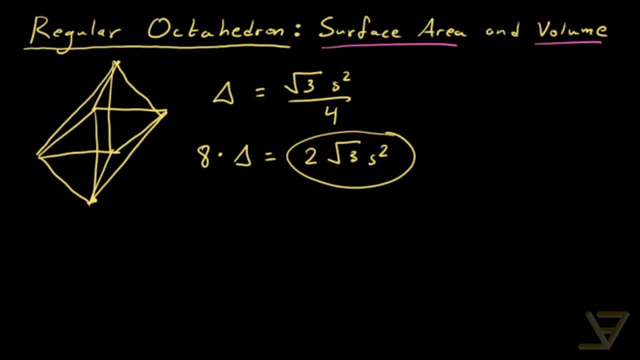 The volume is equal to the volume of the regular octahedron. The volume is equal to the volume of the regular octahedron, So it's just a bit harder. What we have to do is analyze the anatomy of the diagonals of a square. 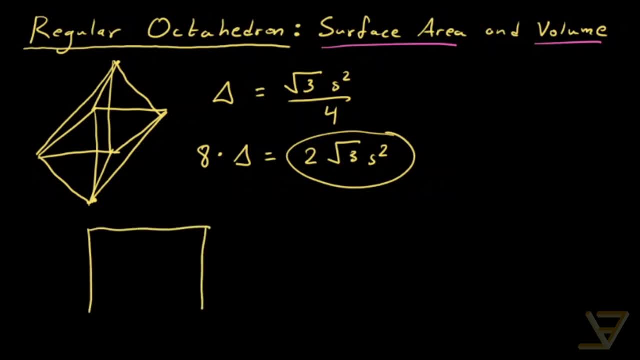 So let's draw a square And then let's draw the diagonals. What we know is that, by the Pythagorean theorem, if the side lengths are s, then the diagonals have length s squared plus s squared square root, square root which is equal to square root of 2s, and so half the diagonal would be that. 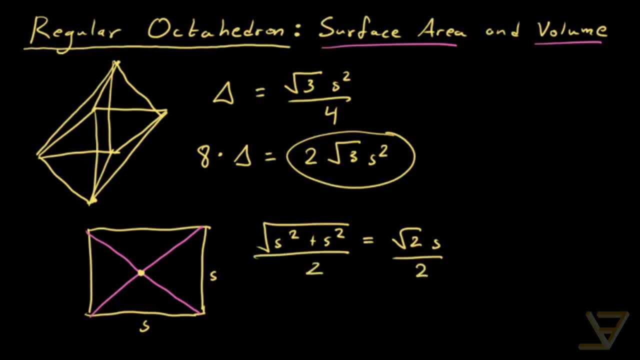 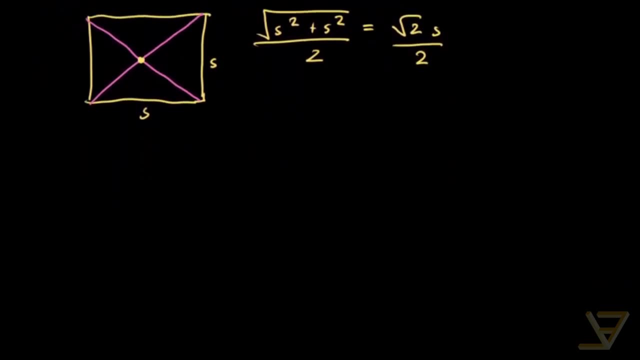 over 2, which is square root of 2s over 2, and what that allows us to do is find the height of the octahedron. So let me draw out an octahedron again. We start with the square, and I'm just going to draw the first one, the one on top. 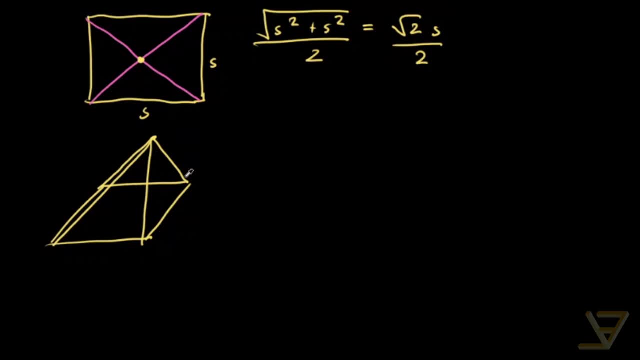 It doesn't look quite regular, but well, let me give it another shot. Let's draw it over here. That looks slightly better, although not that much better, And if we draw the height which goes to the center of the square, then we can find the